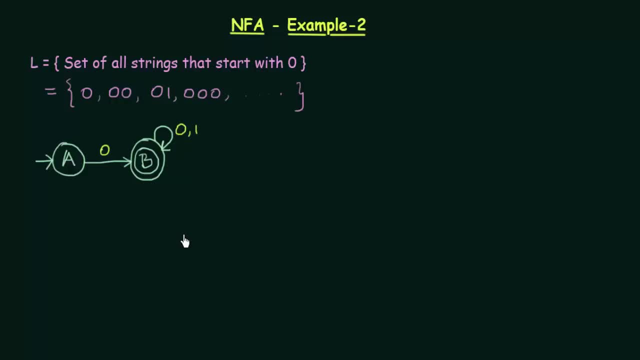 Alright, So here I have completed my NFA. Is it complete? If it was DFA, we could have seen that it is not complete, because we did not mention what happens to A if it gets input 1.. But here I did not mention it. 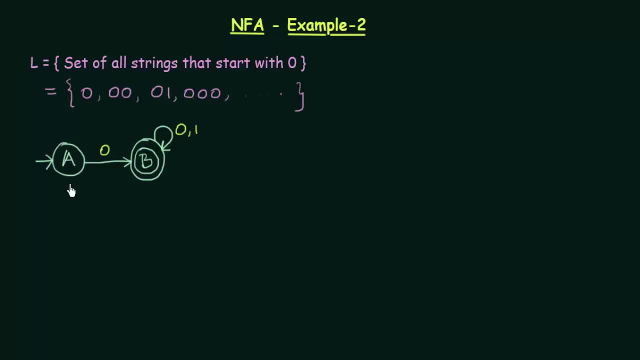 Why? Because this is an NFA And in NFA it does not matter, even if you don't mention that This is a complete NFA. Now let us take a few examples and see what happens. Let me try to pass a few strings. 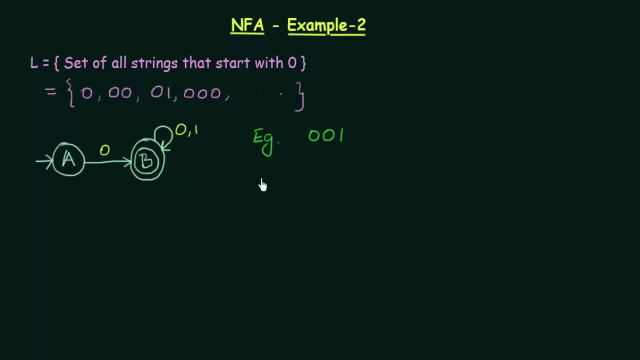 Let me say I will pass this string 001.. So, as usual, I should always start with the starting state, which is my state A And A. on getting input 0, where does it go? It goes to state B. It goes to state B. 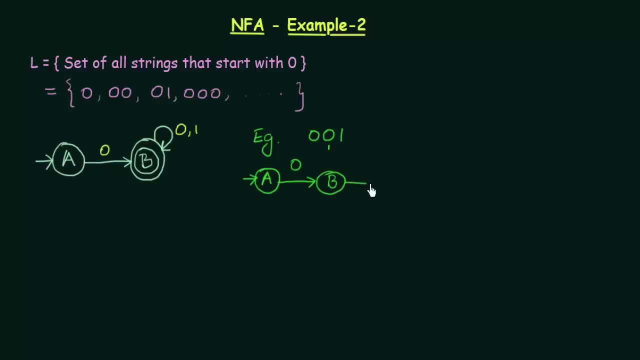 And what is my next input? My next input is again 0.. So B on getting input 0, where does it go? It goes to B itself. It goes to B itself. And what is my next input? My next input is 1.. 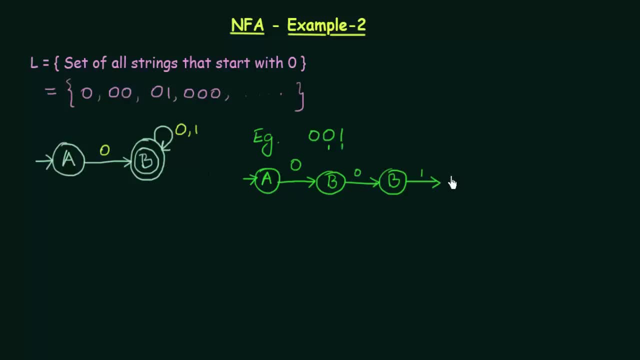 And when B gets input 1, where does it go? It goes to B itself. And now I have reached the end of the string. And at the end of the string, where am I? I am in state B And is state B the final state. 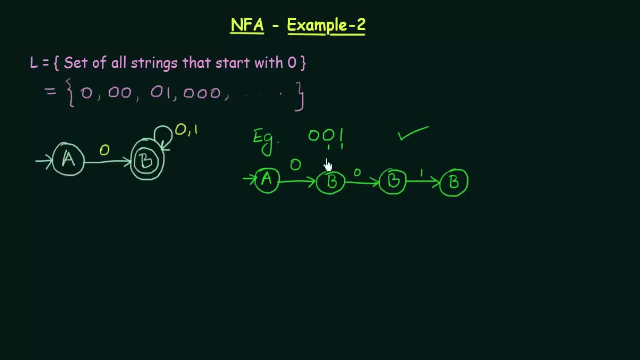 Yes, it is the final state. So this string is accepted. Alright, now let us take another example. In this example, let me test for the string 101.. So I start always with my starting state, which is A And A. on getting input 1, where does it go? 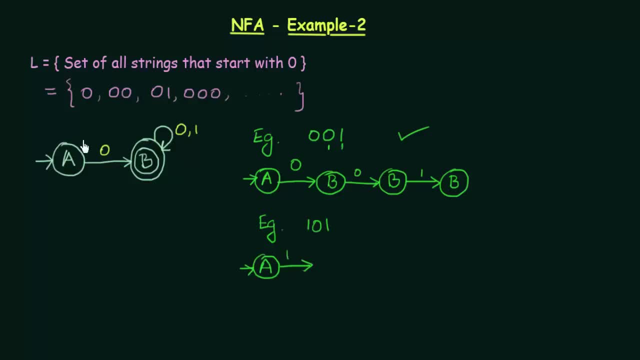 On getting input 1,. A does not have a place to go, So it goes to PHI. I will represent it by PHI. A does not have a place to go. It does not go anywhere. This kind of configuration where a state does not go anywhere. 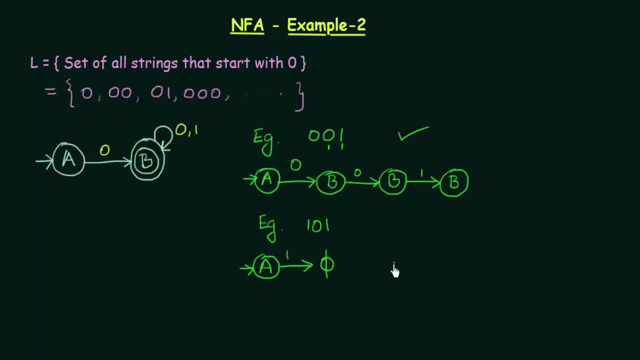 That is known as a dead configuration. That is known as a dead configuration. dead configuration right, okay, but in case of DFA, we did not have a dead configuration. if we leave a DFA like this, this is incomplete. we have to mention where a goes, even if it gets input one. 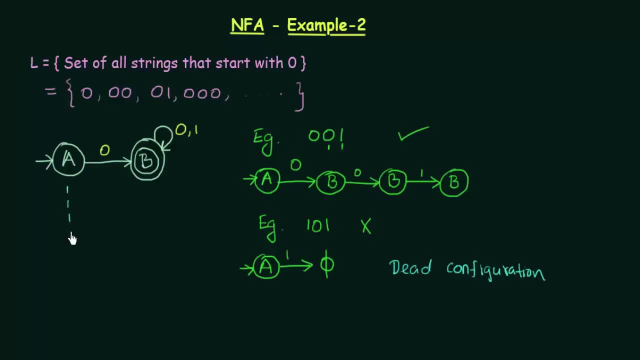 so let me just convert this into a DFA. if I was, if I were to convert it to a DFA, I would send it to another state called state C on getting input one and after coming to state C it stays in state C, whether it gets input zero or one. so from this state C, if a string comes to the state C, it does. 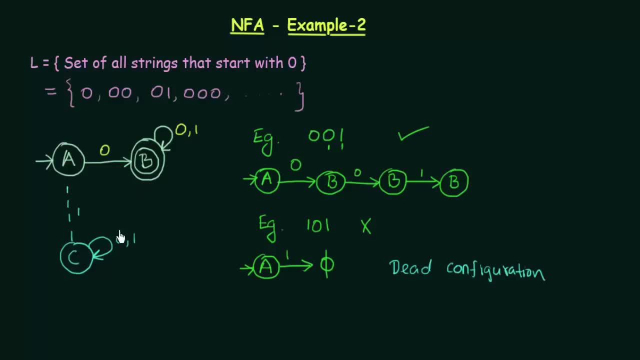 not have any way of going back to this final state B anymore. so in case of our DFA, this state was known as the dead state or the trap state- dead state or trap state. but in case of NFA, we don't need to mention this dead state or trap state. we just leave a the NFA blank, just like this, and 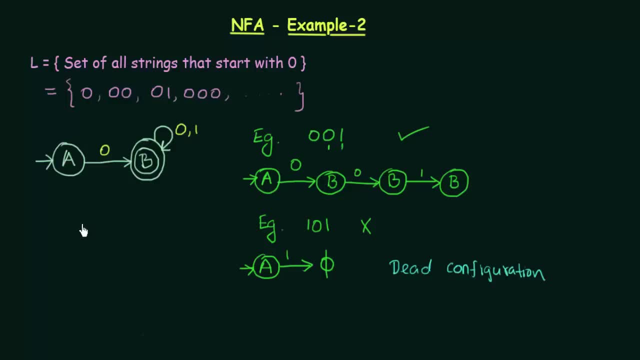 this shows that it is a dead configuration and it is a complete NFA. so this is how to design a NFA, for the set of all strings then starts with zero. okay, now let's see another example: constructor NFA that accepts sets of all strings over zero. 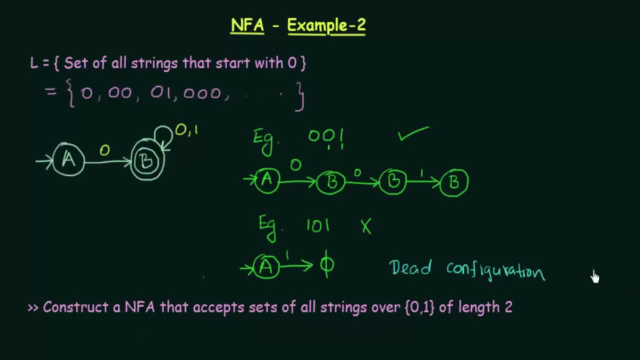 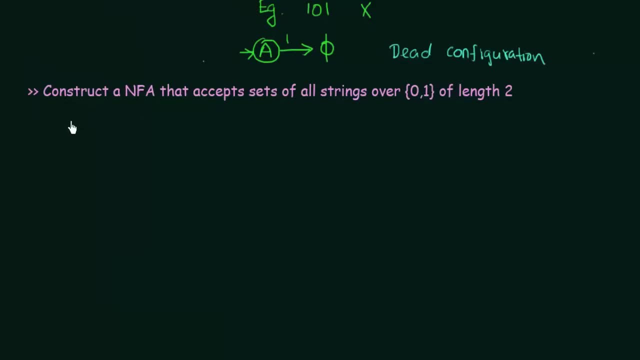 one of length two. so, if you remember, we have done this same thing for DFA as well, so let us see how to construct the NFA for this. so, before starting here, our input symbols are zero and one, and our language. what will be the sets of elements? in our language, it is the sets of all strings over. 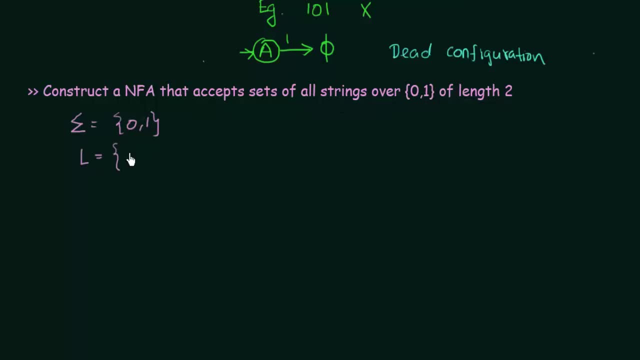 zero one of length two. so what will be the sets of all strings of length two over zero one? they will be zero, zero, zero, one, one zero and one one. okay, now let's see how to construct the NFA for this. it is very simple. first we have- I start with my starting state, which is state a, and then a on. 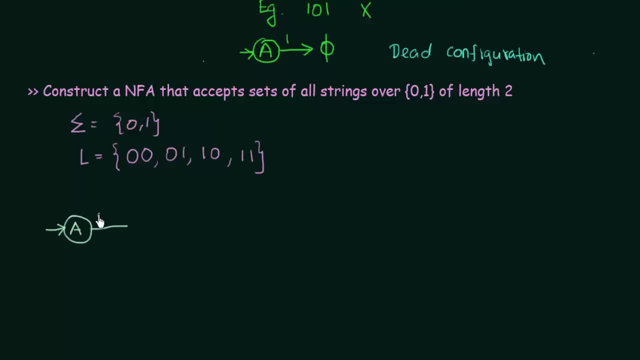 getting input, either zero or one. either zero or one- I send it to state B. and at this point, what is the length of my string? the length of my string is one, right? I just got one input, so I am going to get one input now. on getting the next input, whether it is zero or one, I send it to the next. 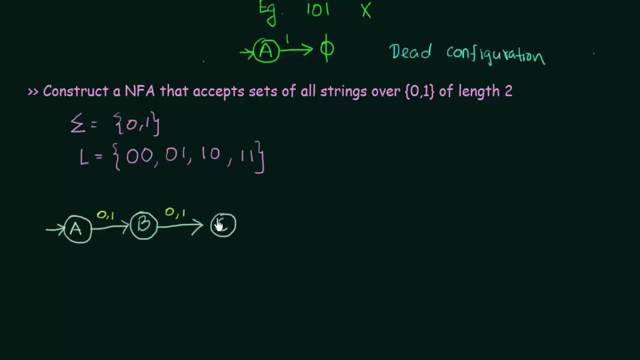 state, which I will call state C. and at this point, what is the length of my string? the length of my string is two. I got my first input here, second input here, so the length of my string is two. so this C should be my final state or accepting state, right? so this is it. this NFA is complete. 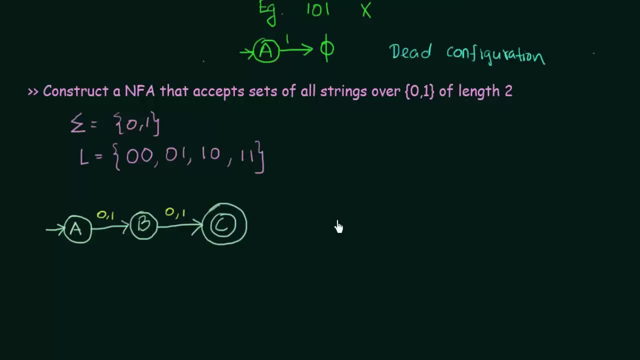 so if it was a DFA, I should have send it to another state here, which will be a trap state or a dead state on getting a next input on state C. but in NFA I don't need to do it. I just leave it like this, showing that this is that configuration means. whatever I get after this state C, it does not go. 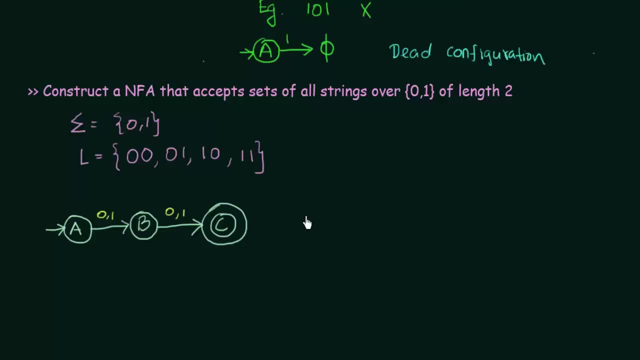 anywhere, so that will be rejected. so let us just take two examples quickly and see how does this work. so let me first check for this string: zero, zero. it should be accepted. so let's see. it starts from state A. on getting input zero, where does it go? it goes to state B and on getting input zero, again, this is the second input. I'm in state. 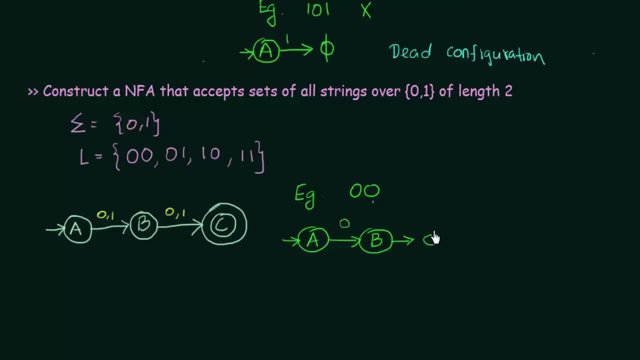 B and I'm getting input zero. where does it go? it goes to state C. and now I resend off the string. and where am I? I am in state C and you see the final state: yes, so this is accepted. okay, so now let's take another example. in this example, I will take the string. 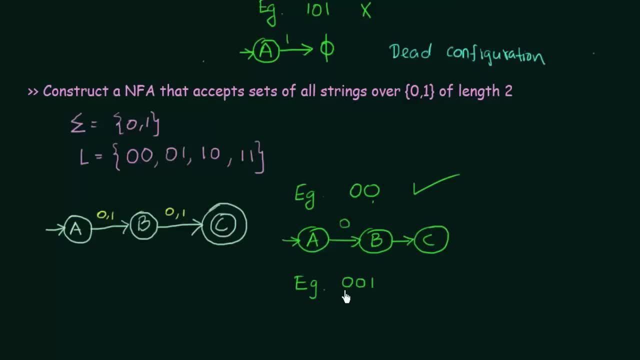 zero, zero, one. now should this be accepted? this should not be accepted. why? because the length of this string is one, two, three and my. the NFA should only accept strings of length two, so let's see whether this should be accepted or not. I start with my starting, state A, and the first input. I 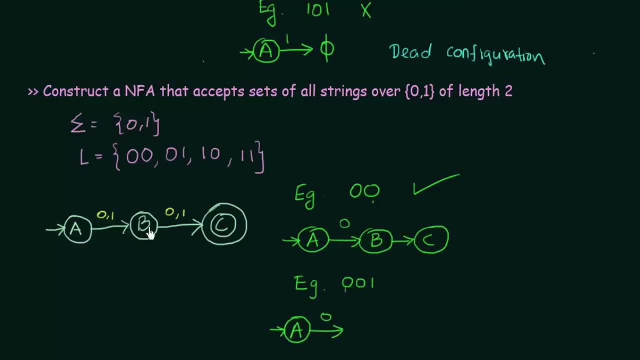 get is zero. so, on getting input zero, where does A go? A goes to B and what is my next input? my next input is zero. so I'm getting this zero. I'm in state B and I'm getting this zero. where does B go? B goes, and now I have the next input, one and C. on getting input one, where does it go? C? on getting input one.